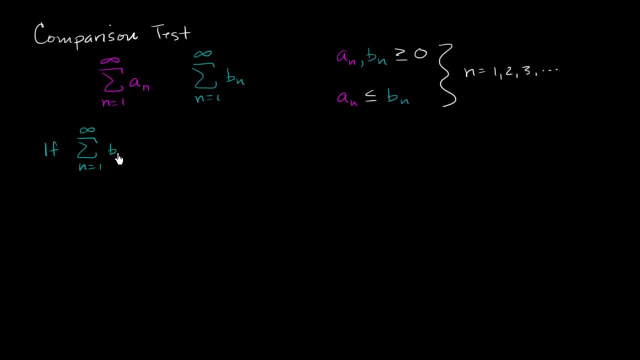 in my brain, the larger series, the one whose corresponding terms are at least as large as the ones here. if this one converges, if this one doesn't go unbounded towards infinity, it goes to, it sums to some finite value. 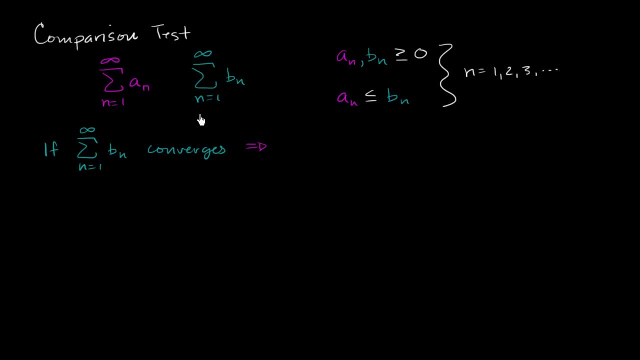 then that tells us that the one that is in some ways- I guess you could say- smaller must also converge. Must also. so this one, this one right over here, must also converge. So that must also converge. So why is that useful? 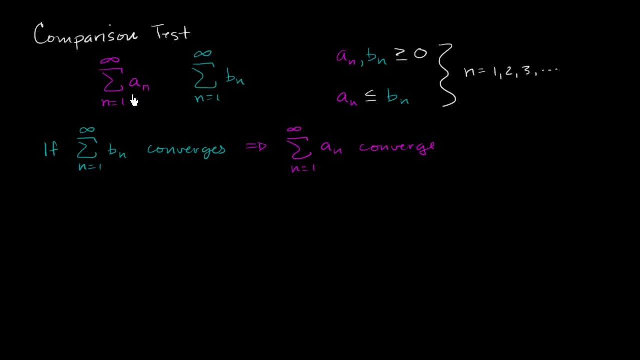 And we'll see this in future videos. Well, if you find, if you're looking, say you have your a sub n and you're like, hey, gee, I wish I could prove that it converges, I kind of have a gut feeling it converges. 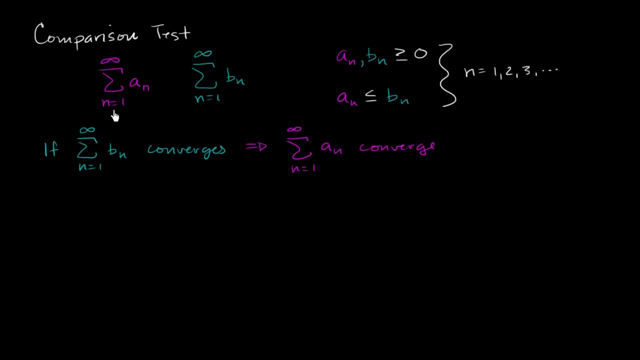 the comparison test tells us: well, just find another series- that is always- whose corresponding terms are at least as large as the corresponding terms here, and if you can prove that one converges, then you're good with this one. And of course it would only apply to the case. 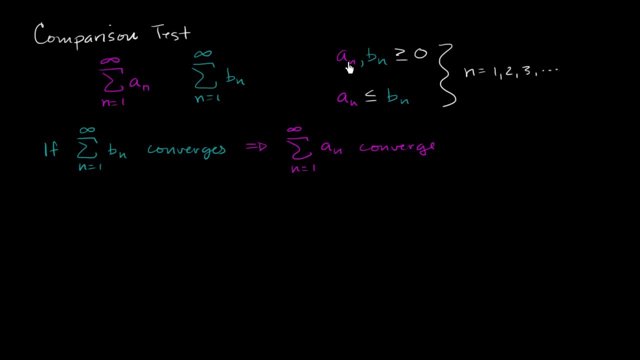 where your original series, each of the terms, each of the terms are non-negative. Now, what if we went the other way around? What if you could prove that the magenta series, the smaller one, and I guess I could kind of put them? 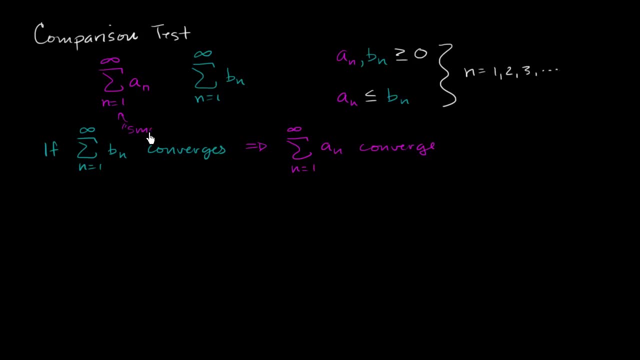 in quotes. you know, this one right over here is: the smaller, the smaller. I guess each of its corresponding terms are smaller. what if you could prove this one diverges? Well, if this one diverges, it's going to go unbounded. 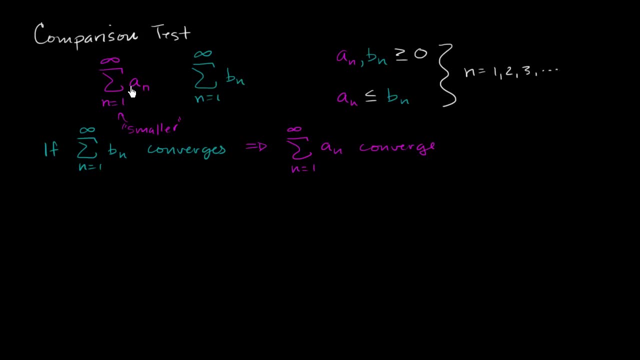 to infinity. it's not going to go to negative infinity. all the terms are positive. it's not going to oscillate. it's not going to diverge because it oscillates between two values. once again, if it's oscillating between values, the only way you could do that. 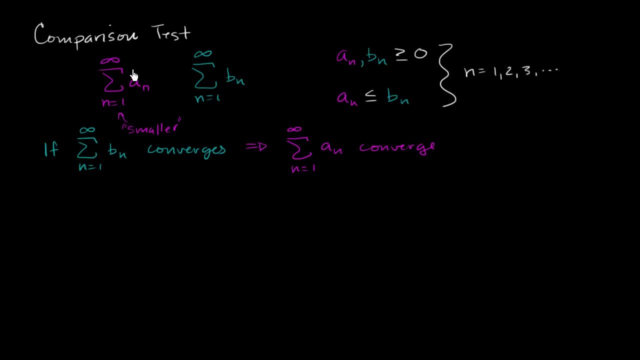 is if you had negative terms here, So this would kind of be unbounded towards infinity. Well, if this one is unbounded, each of these corresponding terms are larger, so this one must also be unbounded. so let's write that down. 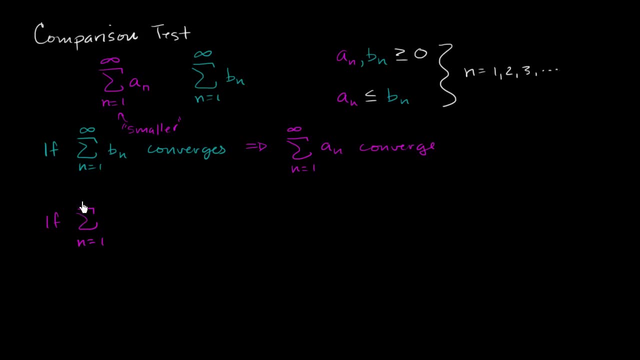 So the comparison test tells us, if our smaller, smaller series diverges, if this one diverges, then the larger one must also diverge, Then the larger one must also diverge. And so, once again, if you wanted to prove that, this thing,